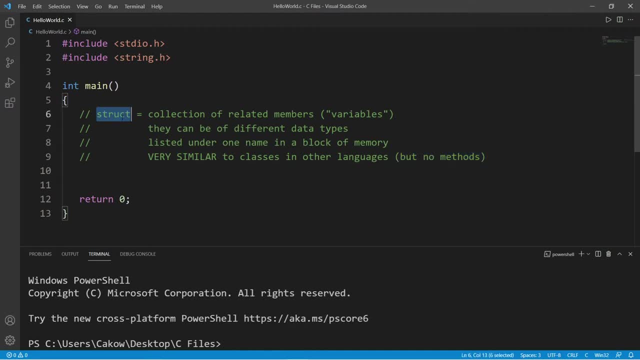 know what a class is, but there are no methods within a struct, It's only members. So we can actually use structs to mimic real-world objects. Let's say that maybe we're playing a game and we need two players. Each player will have a name and a score. These will be 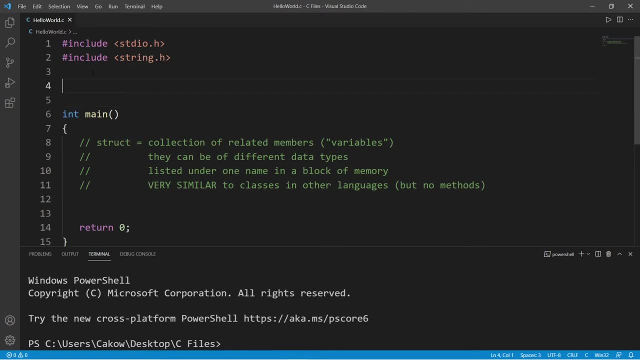 the members. So to create a struct outside of our main function, we will type the keyword struct, followed by a tag name Let's say we are working with. Then we need a set of curly braces, then end it with a semicolon. So any members think. 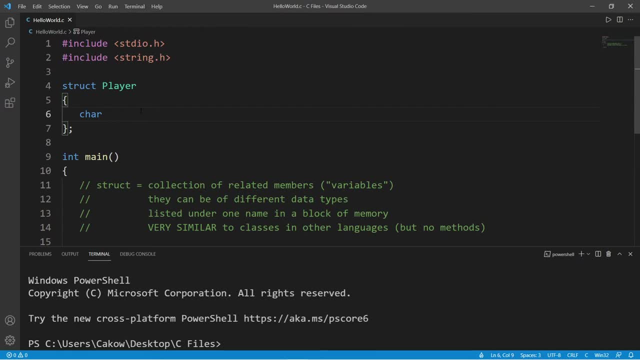 of these like variables. So let's say we have a character array named name, and I'll give this a size of maybe 12. So we will declare these but not assign them- We'll do that later- And we have an int named score. So each player is going to have a name and a score, kind. 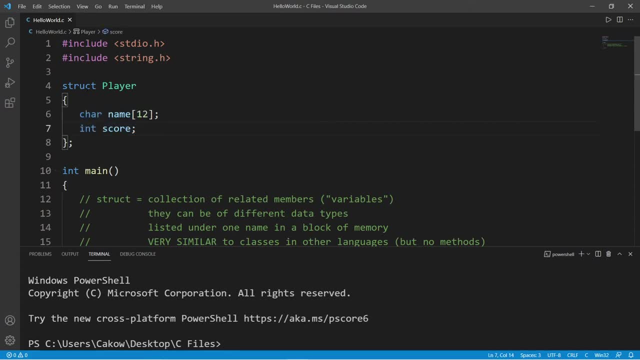 of like we're playing an arcade game. Now, to assign some of these values, we're going to create a type of variable and we're going to think of a player. Let's say it's the same thing as the string And the number. 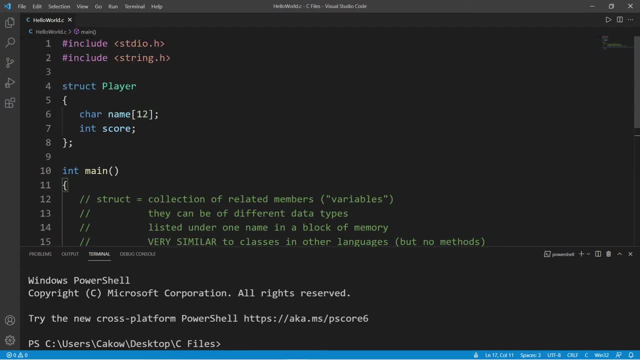 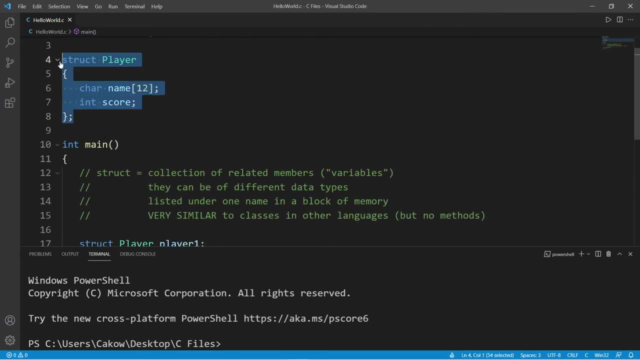 of fighters is 2.. Now we're going to introduce a star and we're going to add to it all of these values And instead of 3, then we'll add 1.. So we'll add one number to the space and we'll give it a variable and a player instead. 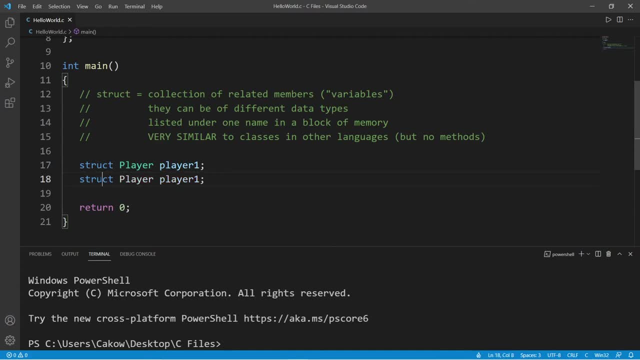 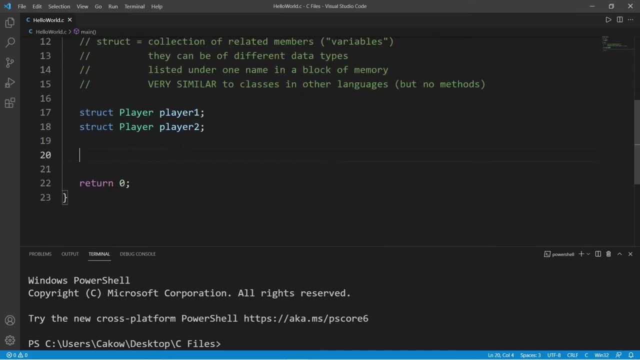 of 3, we two come from 1. And the player worldITAWS. so we're going to add to these values, we're going to add to thisила, So I will call it a various illustrations. Another good way to say this is this: and next I'm going to drag this up- This is going to 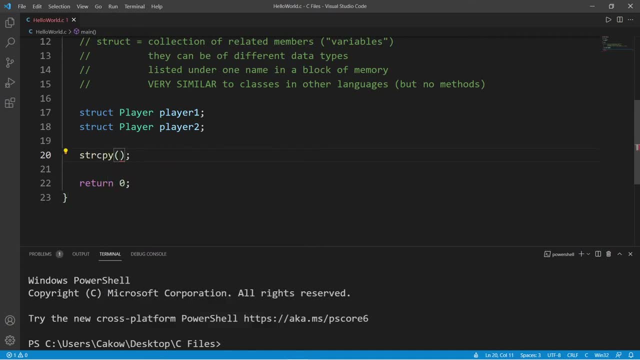 copy function. Then, to access one of the members, you will type the name of that struct. So let's say player one and then follow this with a dot. The dot is a member access operator. So after typing the dot we have access to a name and score member. So let's set the player's name equal to. 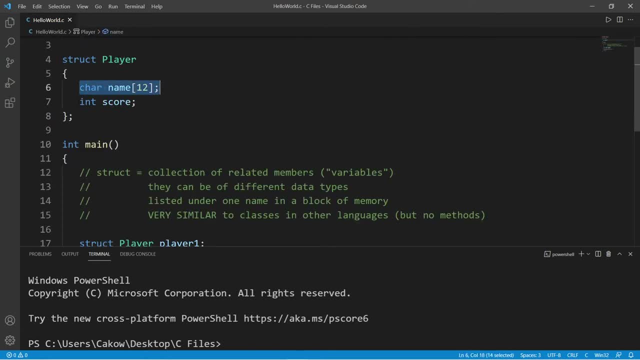 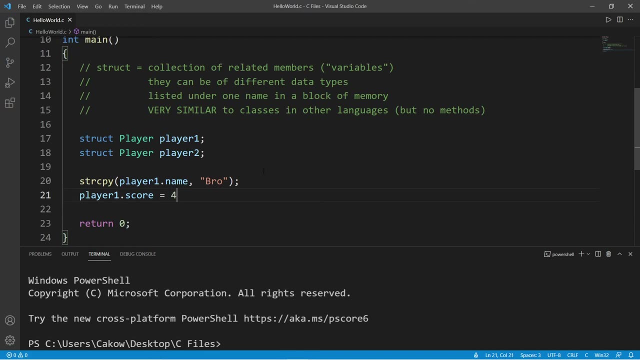 whatever your first name is. Now, if you're not working with an array of characters, such as an integer, you can just access these directly. So let's set player one's score to equal maybe four points. And we also have player two, but we have not assigned values to its members, So this time,